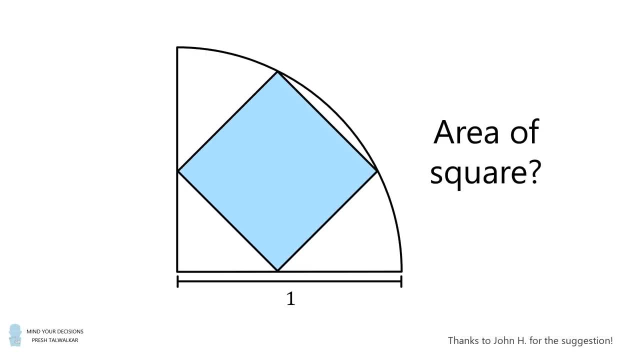 12 to 13 years old. I think it's a very challenging problem to give to students of that age group and in fact, I think many geometry students would find this to be a challenging problem. Pause the video if you'd like to give this problem a try. 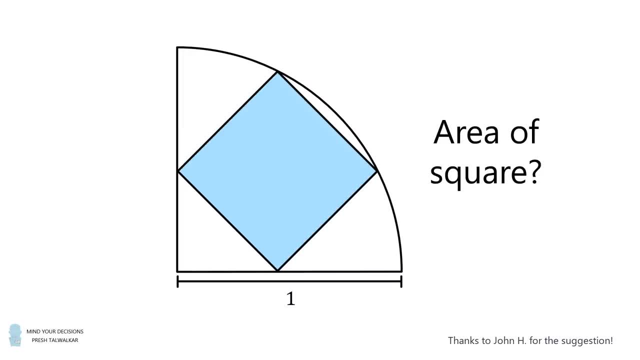 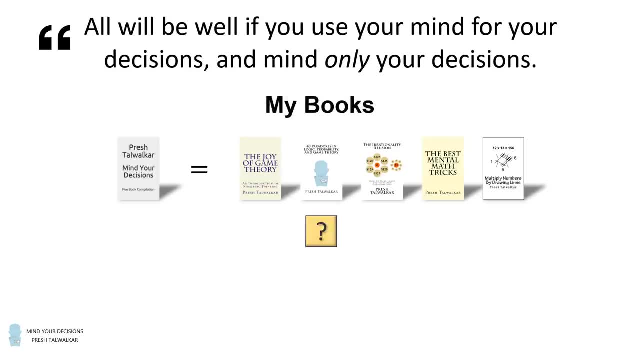 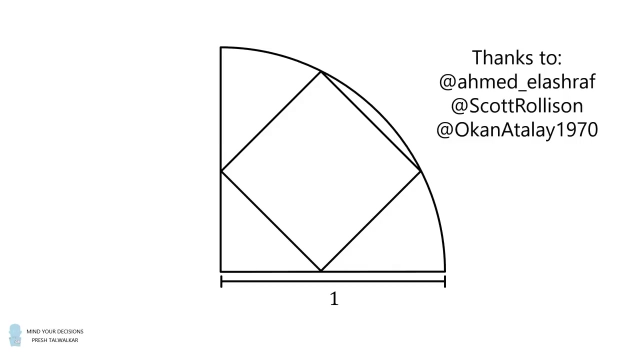 and, when you're ready, keep watching to learn how to solve this problem Before I present the solution. I would like to thank the following people who helped me solve this problem on Twitter, Thanks to at: Ahmed underscore Elashrof, at Scott Rawlinson and at 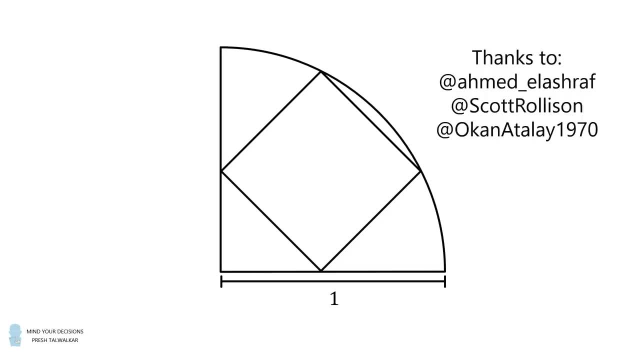 Oken Atalay1970.. To solve this problem, consider the side of the square that's a chord of the quarter circle. Construct a square that's a chord of the quarter circle and then add a square that's a perpendicular bisector of this chord. Since it's a perpendicular bisector of a chord, 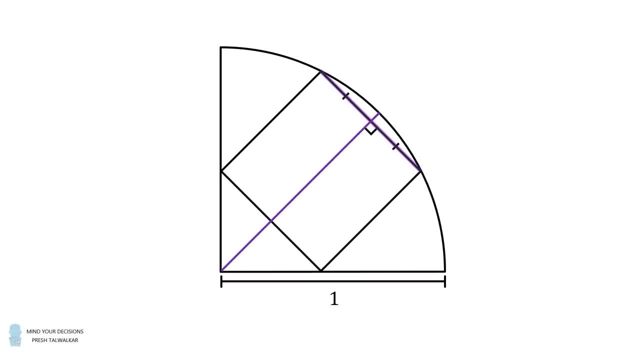 it will pass through the center of the quarter circle. Then, since we have a square, this will also be the perpendicular bisector of the opposite side of the square. Now consider this right triangle By side-angle-side. we will have a congruent right triangle right next to it. 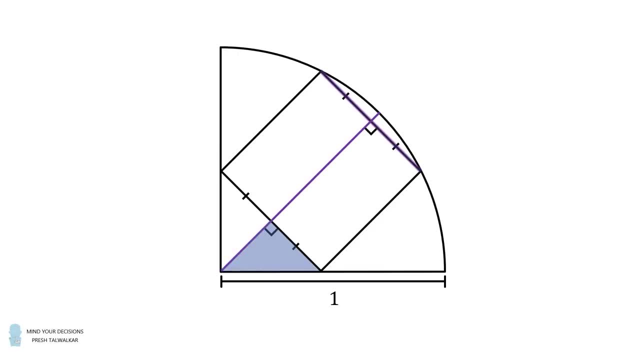 Since these two triangles are congruent, they will bisect the 90 degrees of the quarter circle. In other words, these two angles will each be equal to 45 degrees. Then this means each of these triangles is an isosceles right triangle. 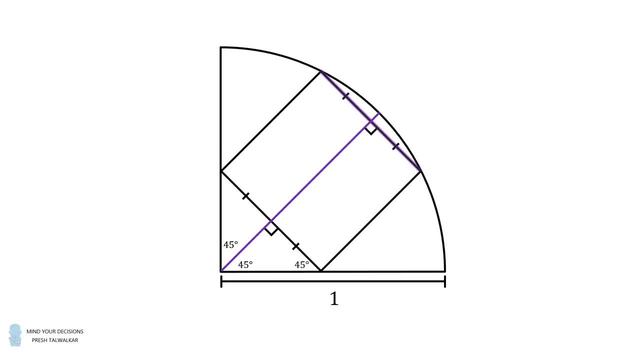 where each of the acute angles is equal to 45 degrees and therefore the two legs of these right triangles are equal to each other. So this distance is also equal to the other leg of the right triangle. We will now use this information to solve the problem. Let's remove some of these markings. 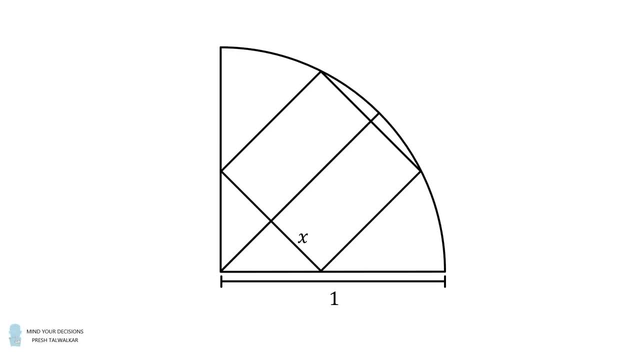 Suppose half the side of the square has a length equal to x, Then these distances will also be equal to x and the side of the square will be equal to 2x. Now construct this radius of the circle. Since it's a radius of the circle, its length will be equal to 1.. Now consider this right triangle.